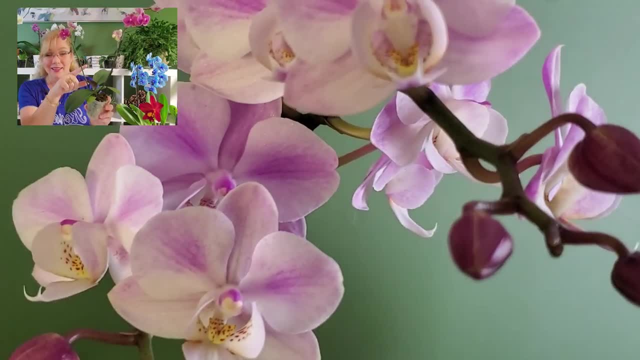 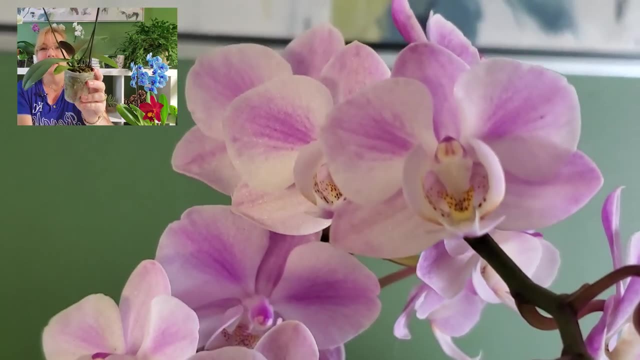 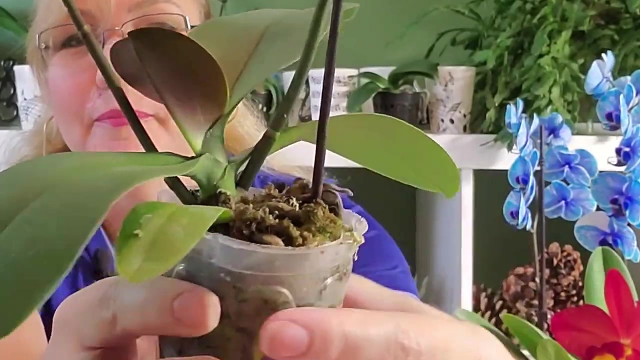 Phalaenopsis will not emerge from the center. That's what's going to make it different from a Paphiopedilum: It's going to emerge from the side. Now, if you look here, you can see the flower spike is emerging from the side of the stem. on this side too, It's emerging from the side. 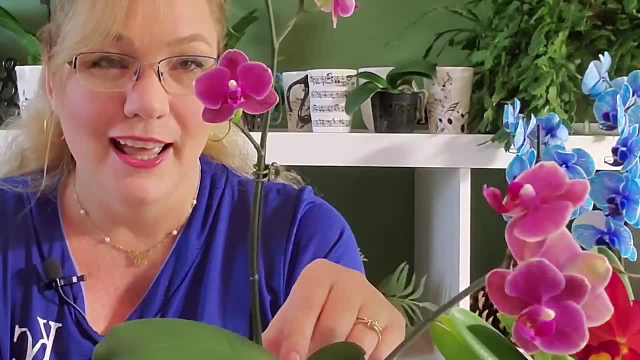 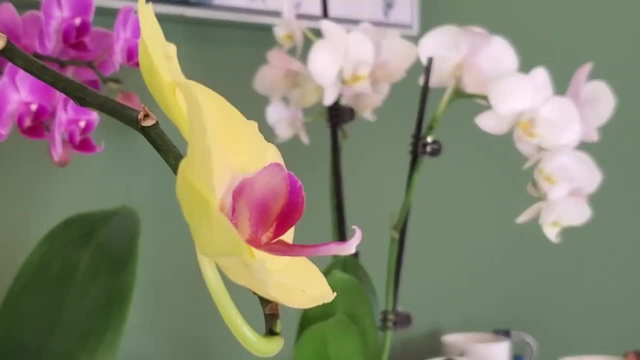 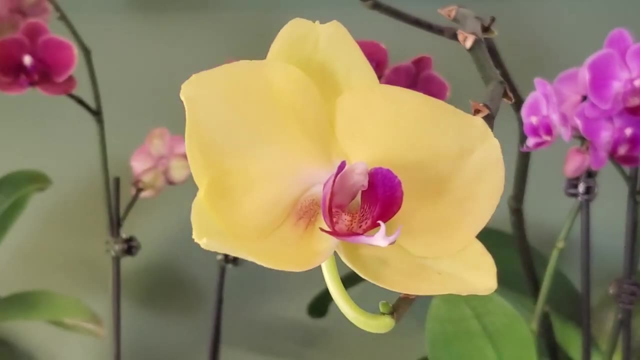 If a flower spike emerges from the center and it still has these kind of flowers, then what you have is a terminal spike on your Phalaenopsis. Phalaenopsis orchids will have aerial roots, and some other plants that have this kind of leaf formation will not Now this one. that 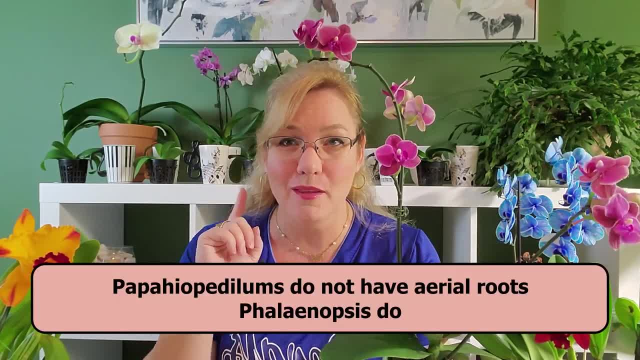 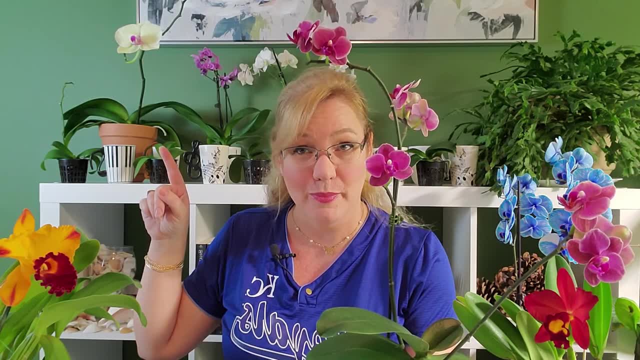 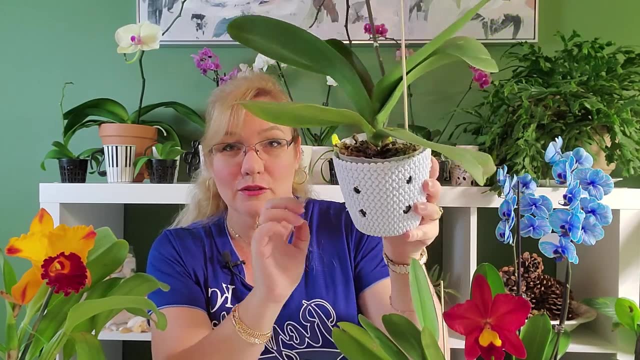 right here does not have aerial roots. but if you look at this huge Phalaenopsis here and right there, it's a little aerial root that is popping out of the pot. There's the main stem of the orchid and one leaf to the left, one leaf to the right. Now this is an adult Phalaenopsis, but there are 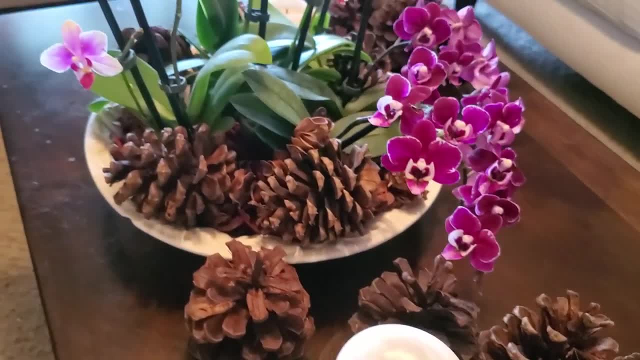 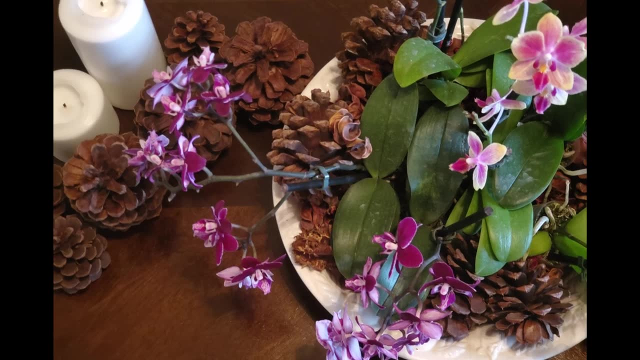 many Phalaenopsis also which are adults in their complete size. This is also an adult Phalaenopsis. It's just a mini and this is the only Phalaenopsis I have, So don't be confused about the size. Just look at the difference. 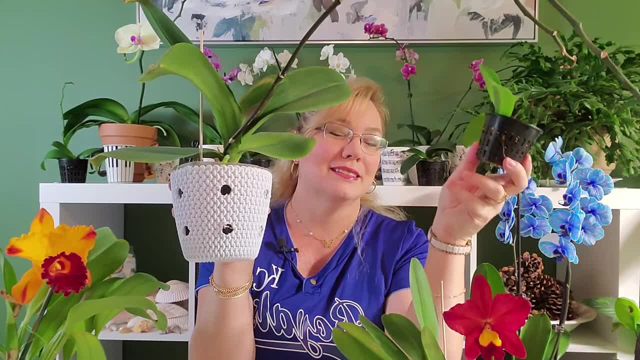 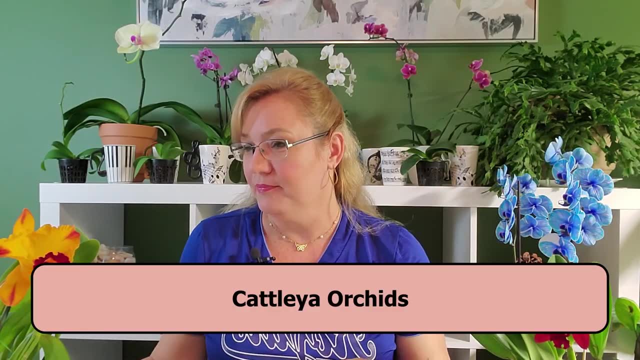 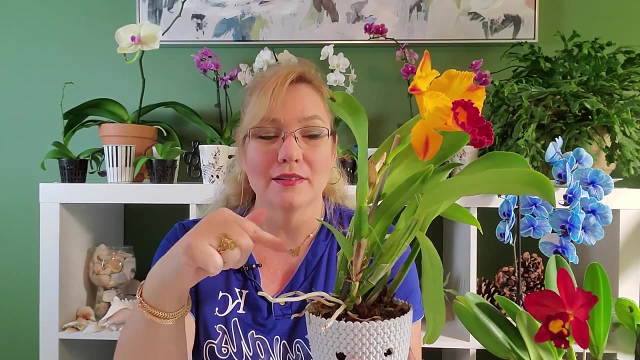 I mean, look at that, and the flower spike just goes all the way over to the end of the video. The second group of orchids are the Catlea orchids. Now, this is a Catlea orchid and, as you can tell, there is not one central stem, There are several stems, and this is what I was talking about. 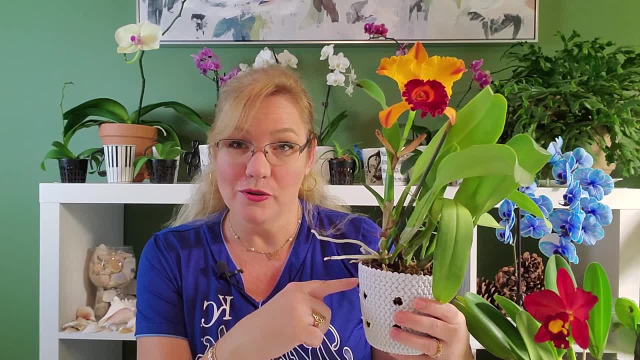 aerial roots here. This is an adult Phalaenopsis. This is an adult Phalaenopsis. This is an adult Phalaenopsis. This is a great example. Catlea orchids will have one horizontal rhizome and from there there's. 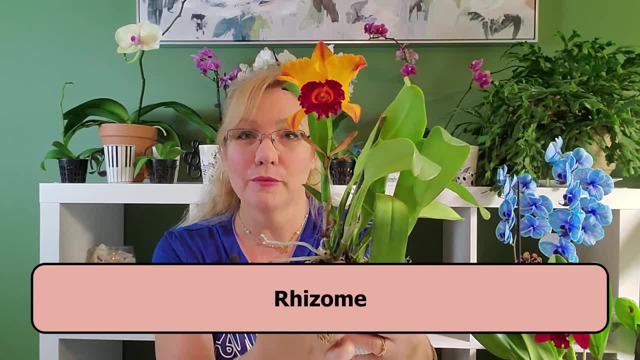 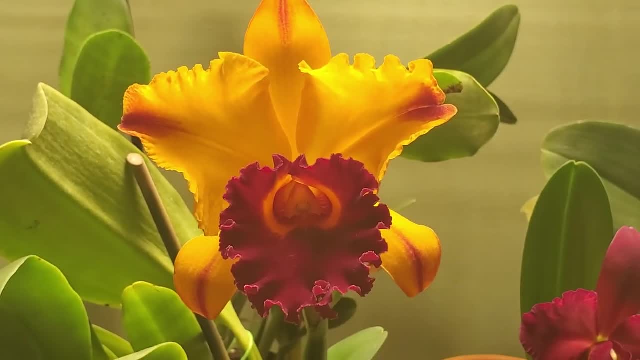 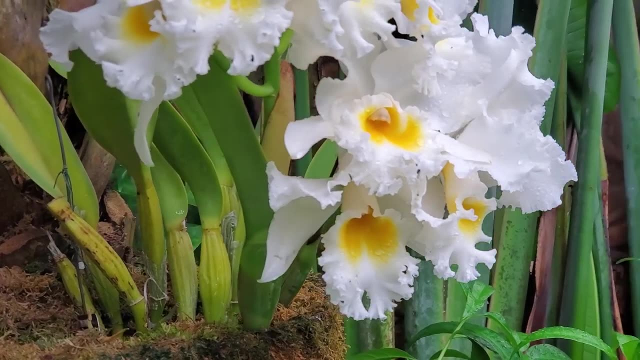 going to be different pseudobulbs that sprout up from the rhizome. So it is a bushier plant and it grows horizontally, not vertically, and the flower, as you can tell, does not grow in one flower spike with a lot of different flowers. It will have one spike with one flower on each of these. 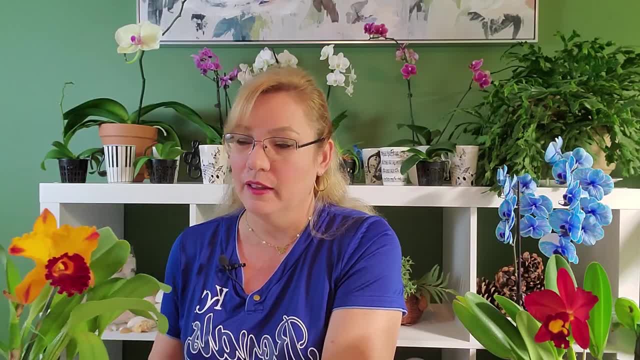 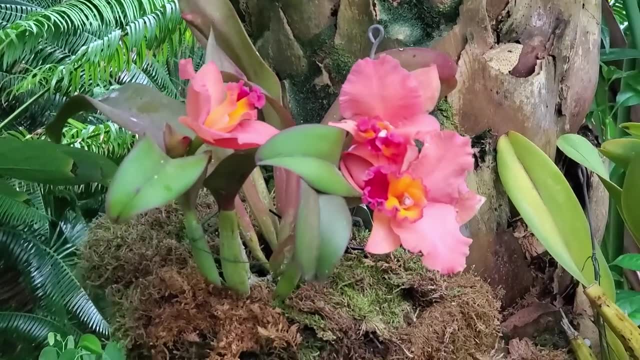 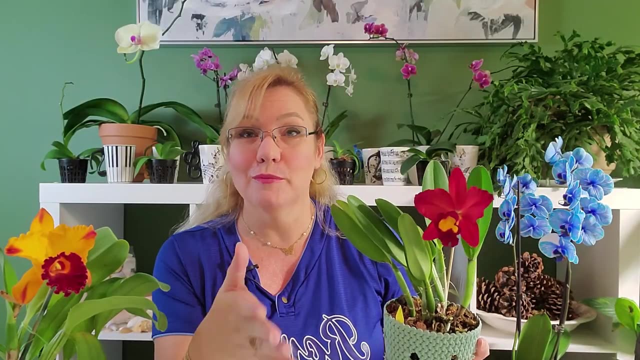 bulbs that are producing, that are in active growth. Here is another Catlea. Catleas can come in all sizes. They can come in miniature too. For the longest time the Catlea orchid was produced for corsages and they were the number one selling orchid. They stay in bloom for about three to 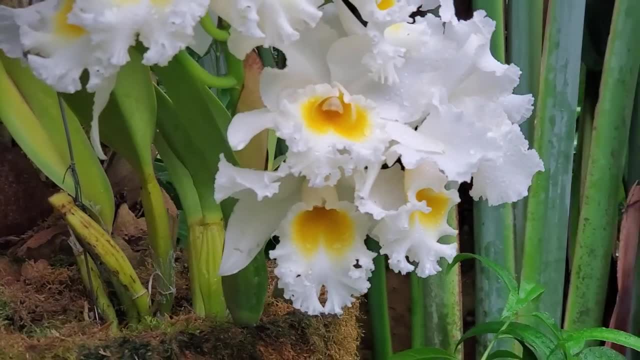 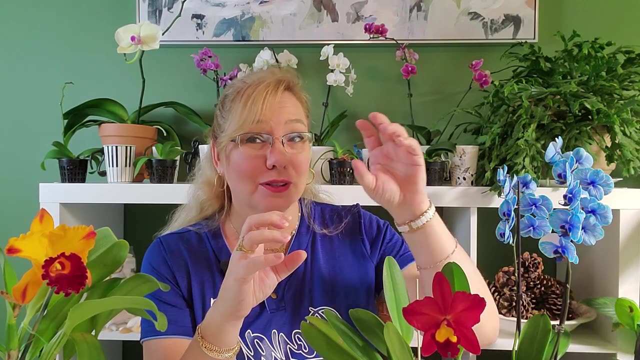 four weeks, but the Phalaenopsis orchid will stay in bloom from the beginning blossom all the way down to the last year or so. So this is a great example of the Phalaenopsis orchid. This is a perfect example of the Phalaenopsis orchid. There's a really amazing 다음or, One in six. 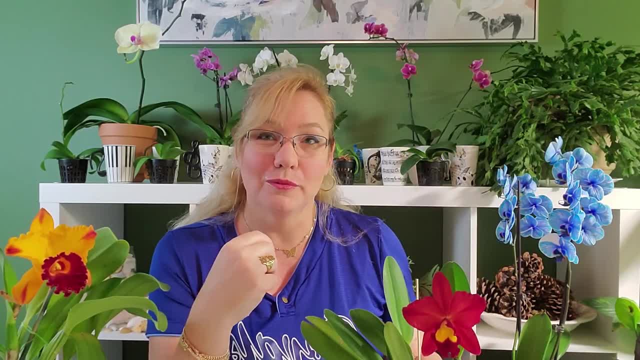 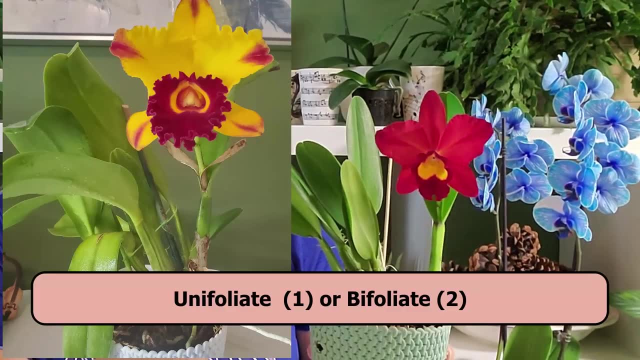 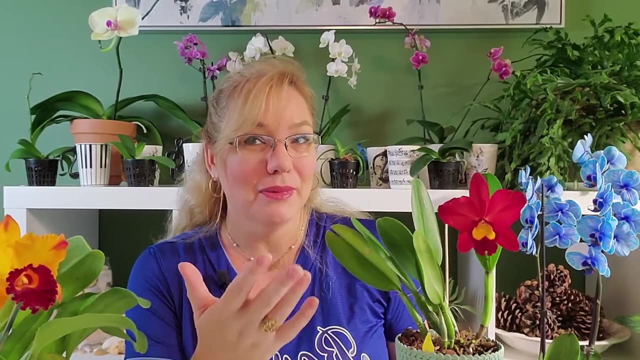 months will start growing. from this previous variety, This was the last blossom on the spike. It can be up to three months, So that is why the Phalaenopsis got a head start on being the number one produced orchid in the world. Catleas can come with one pseudobulb and one leaf, which is called. 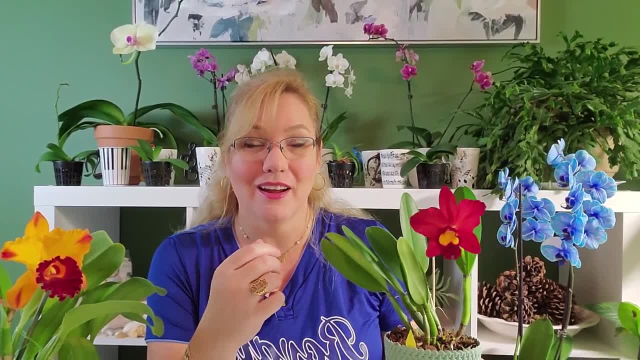 unifoliate, or one pseudobulb, and branch out in two leaves, which is called bifoliate. Now, this doesn't make them any different. They are still Catleas. They just are a different kind of Catleas. Our third orcid is papillotorps. 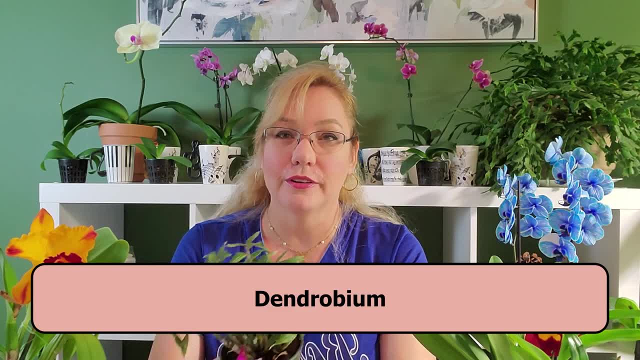 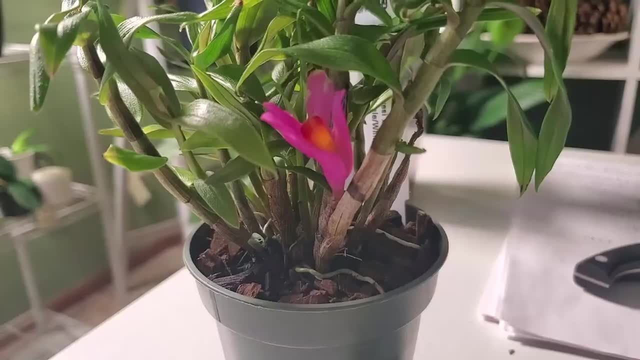 is the dendrobium orchid. now I have two here that are very different. this is a smaller, shorter one, and you can see it grows from a rhizome and has different little canes all the way around. the cane is another word for a suitable and you. 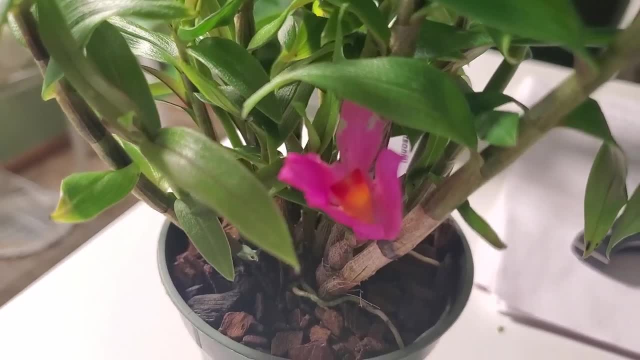 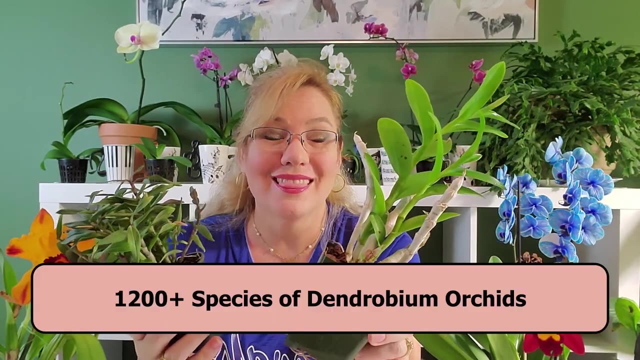 can always tell a dendrobium because their leaves are longer than they are wider. here is another dendrobium. now look at the difference, see dendrobiums. there are more than 1,200 types of dendrobiums. these are just two, so you. 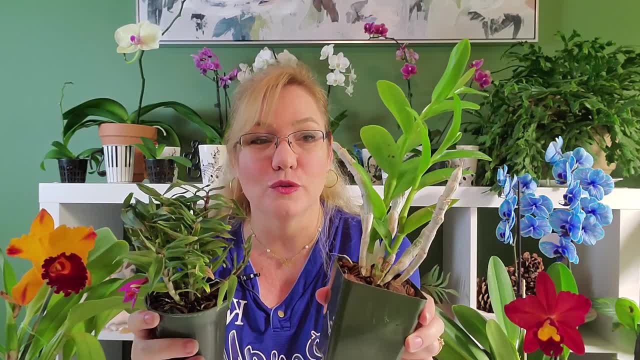 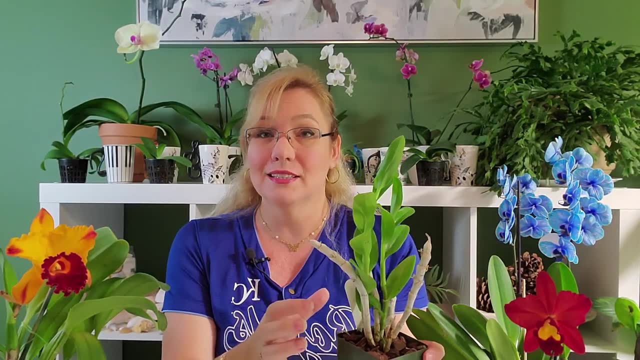 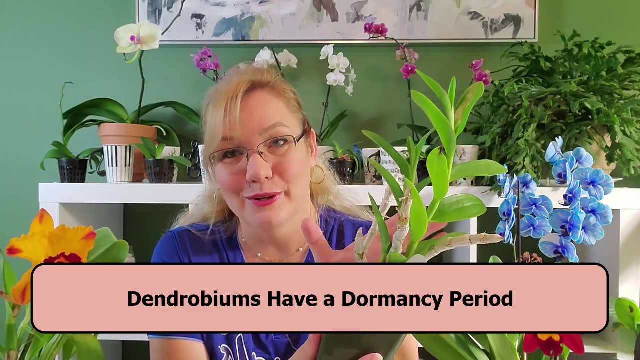 can see how different the care is in each one of these, a dendrobium orchid. you can tell easily because after this flowers, all these leaves are gonna fall off and this is gonna be the ugliest little orchid you've ever bought and you're gonna want to throw it in the trash. please don't, it's just going. 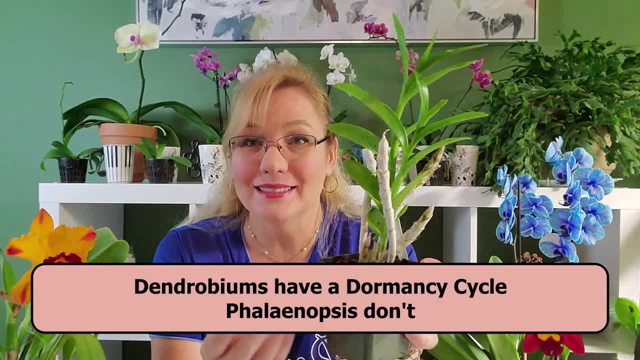 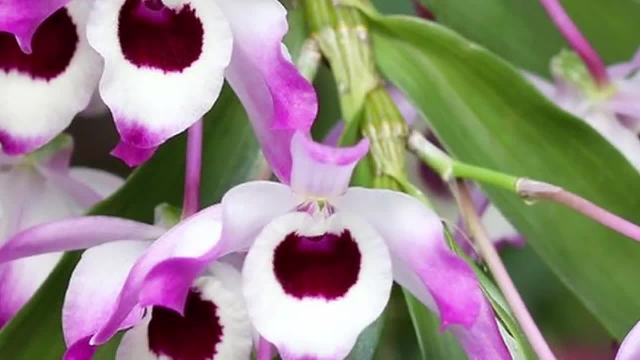 through a dormancy cycle, and on the dormancy cycle it needs to save as much energy as it can so it can produce on that next year a beautiful flower. So if you get an orchid where this dust has these ugly little canes, take your time. 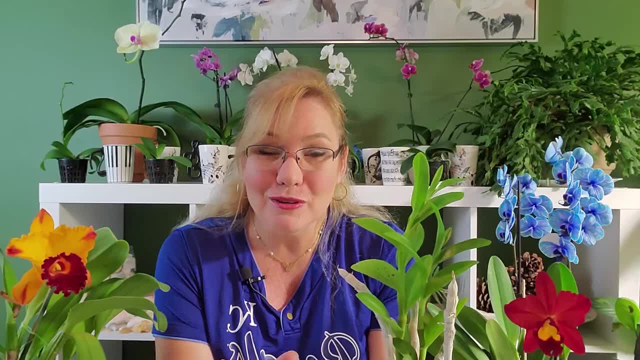 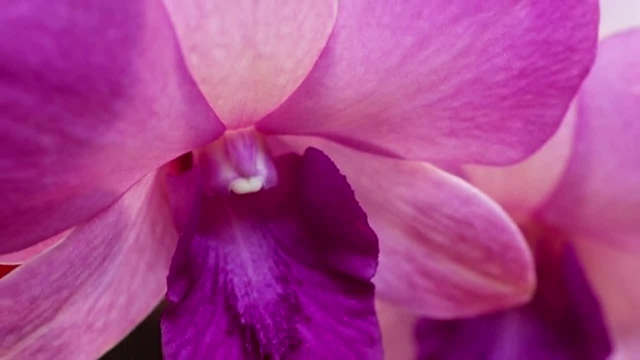 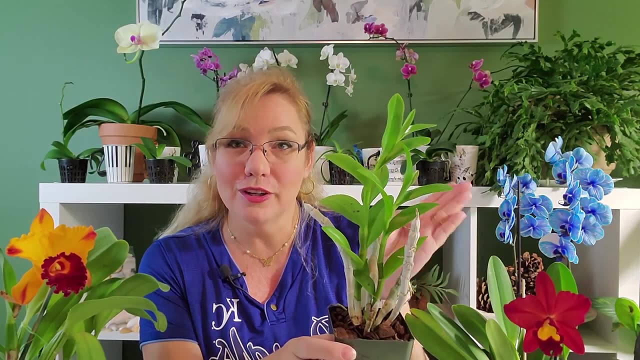 relax When all the leaves fall off. you know, just go slow, Your dendrobium will come back to life later. Now to differentiate a dendrobium from a Phalaenopsis. first you'll notice the stem doesn't stay short. It's always going to be a little longer, Even though there is one leaf to. 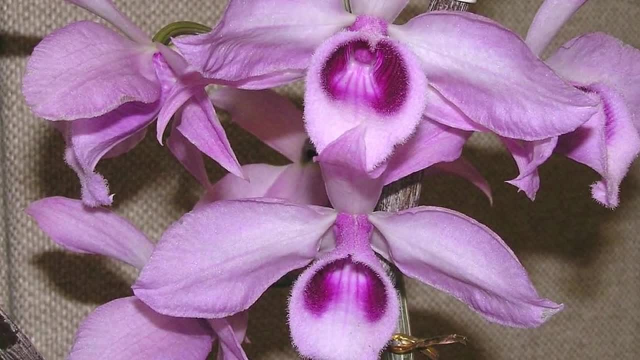 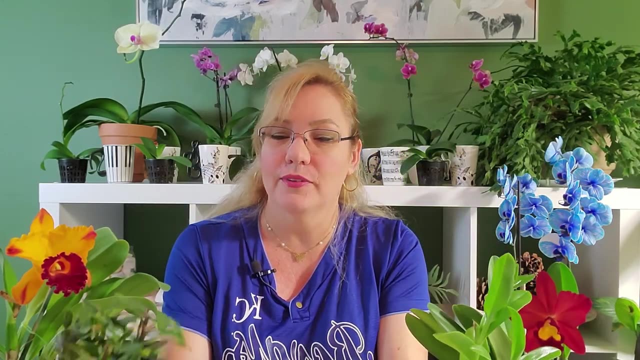 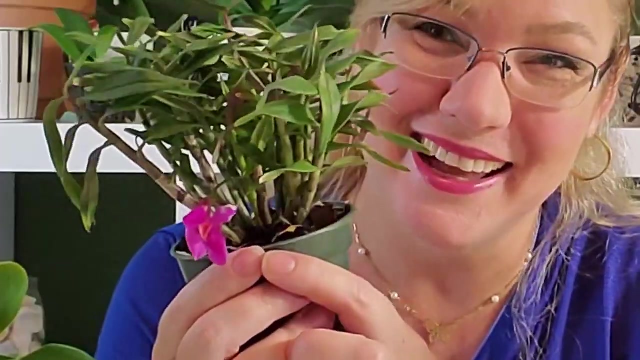 the left, one leaf to the right, one leaf to the left, one leaf to the right. space in between the leaves are extensively longer on the stem, And this is for both types of Phalaenopsis. It's always one leaf to the left, one leaf to the right, And this one's in bloom. Isn't that cute? Oh, it's just. 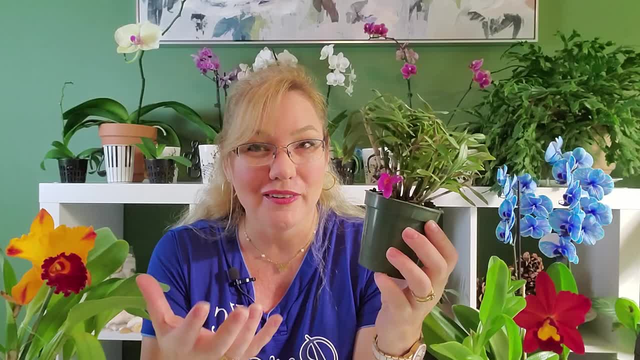 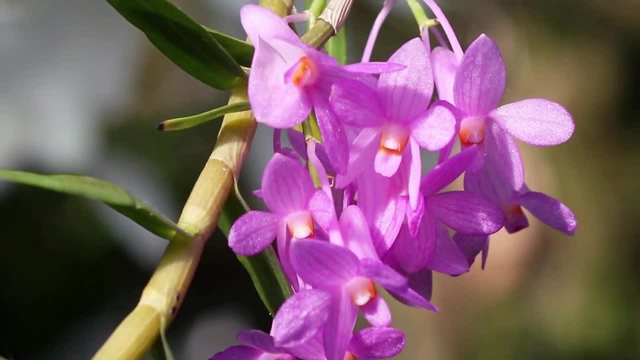 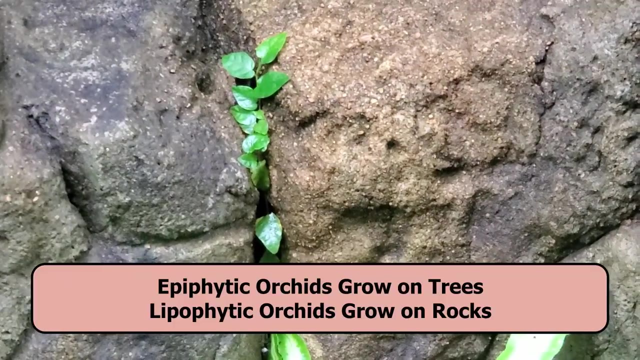 so That's what I love about orchids: They're so varied, They're so different from each other, which makes their care also very different. Don't put all dendrobium orchids in the same category. Some are epithytes and they'll grow on trees, Others are terrestrial and will. 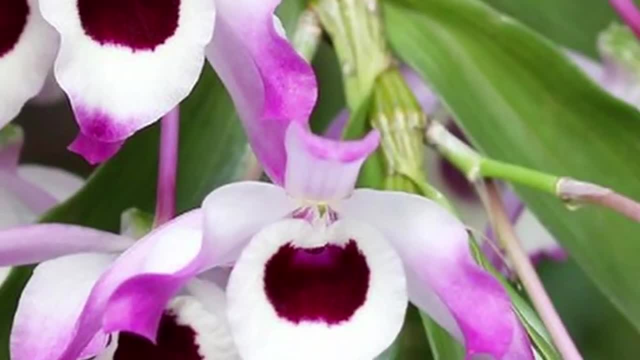 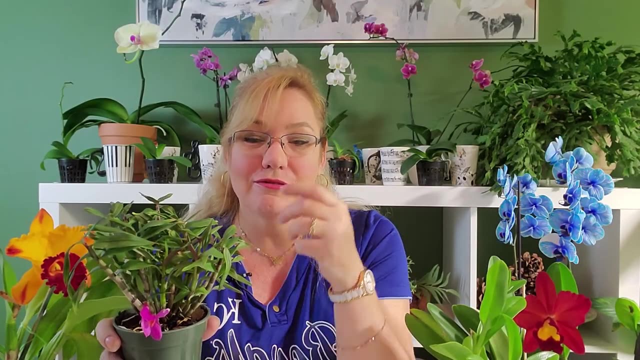 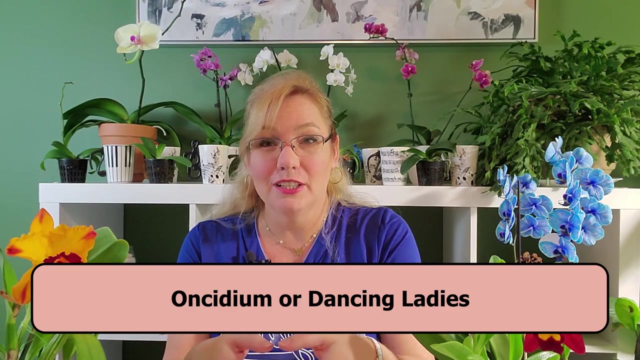 grow in a potting mix that resembles a leaf litter, So you need to really research your dendrobium and find out more about it. Our fourth group of orchids are the Oncidiums. Now, at the time of this video, I don't have an Oncidium with me, but Oncidiums are extremely beautiful. 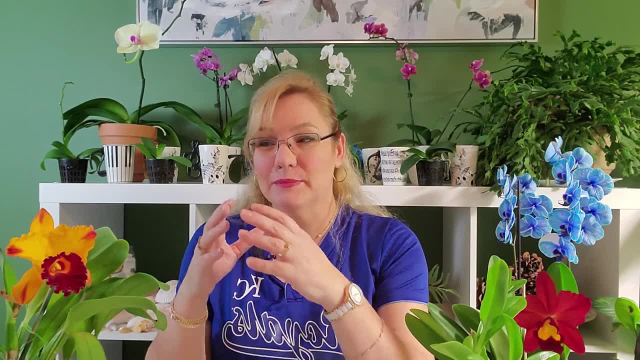 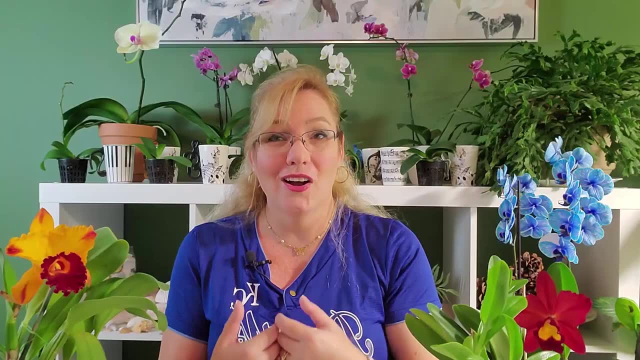 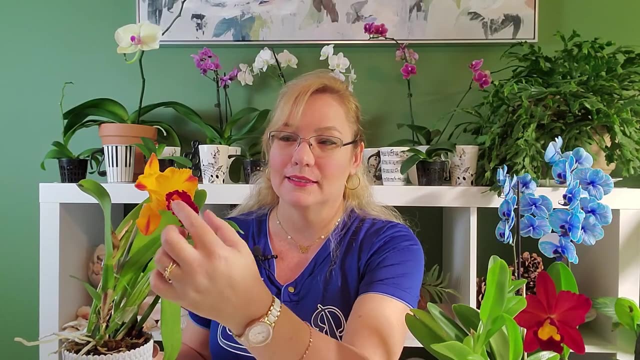 orchids. They're called dancing ladies, and that is because they will blossom, and on each blossom they'll have multiple flowers that cascade down. Oncidiums get this name because their lip, or labellum, which is this part of the orchid, this one petal, as I can call it, is extremely 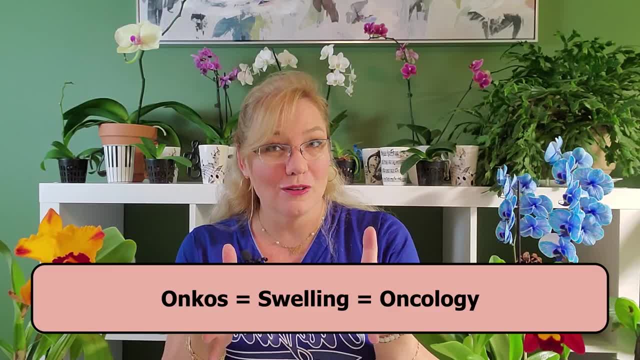 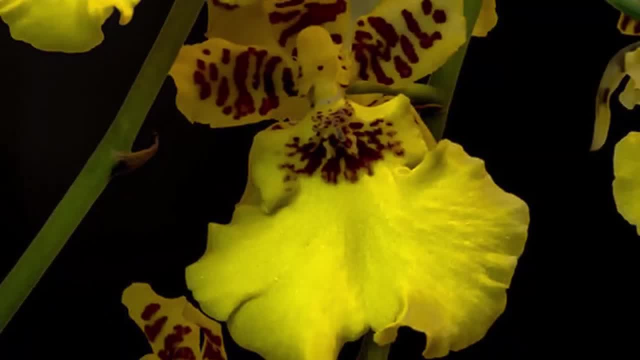 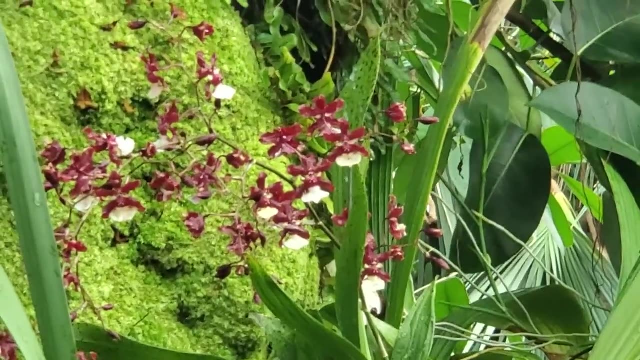 enlarged. This swelling is called Oncos, which is also where we get our word Oncology, because of the swelling of the cancer cells. They can be mainly yellow or red and they have a beautiful fragrance. The most famous Oncidium is not yellow, but it's famous for its smell because it has a 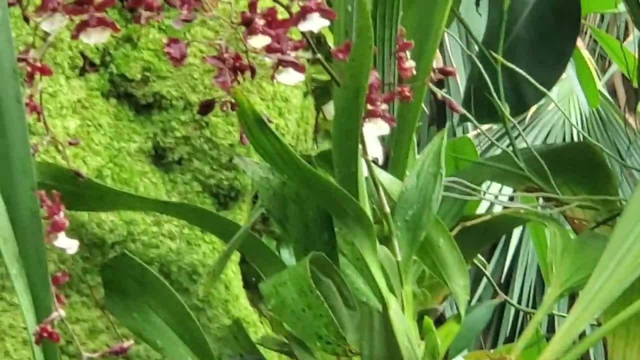 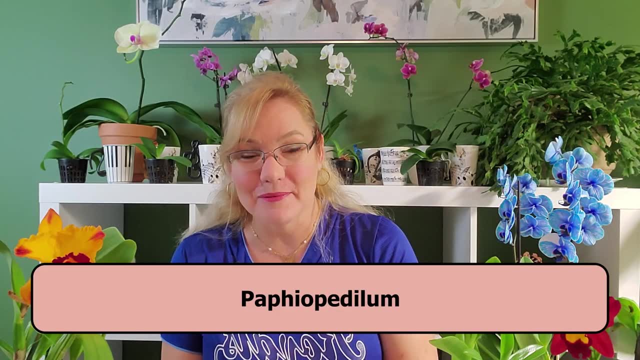 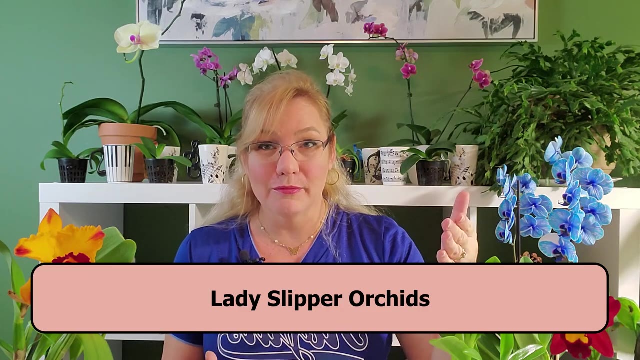 chocolate smell to it And it is just so enticing called an Oncidium Sherry Baby. fifth group of orchids are called the pathiopedilums. Now, pathiopedilums are commonly called the lady slipper orchids, but lady slippers also include phragmopediums and other types of orchids too. 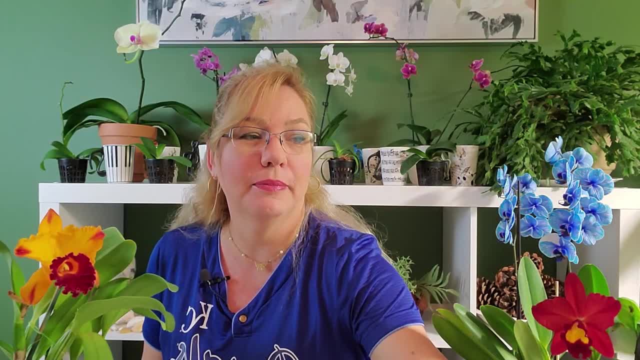 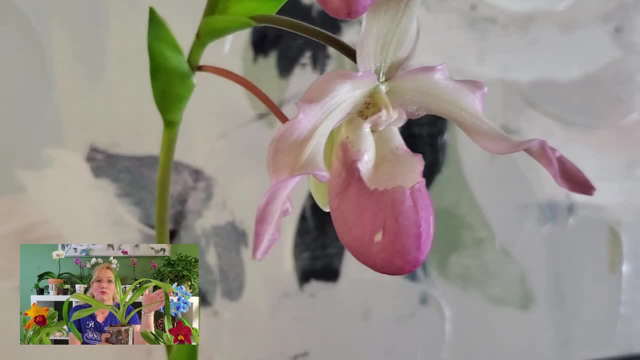 I don't have a pathiopedilum, but I do have a phragmopedium and it's not in bloom. but you can tell the size of this thing. I mean, it's huge. and it does have one to the left, one to the right, but 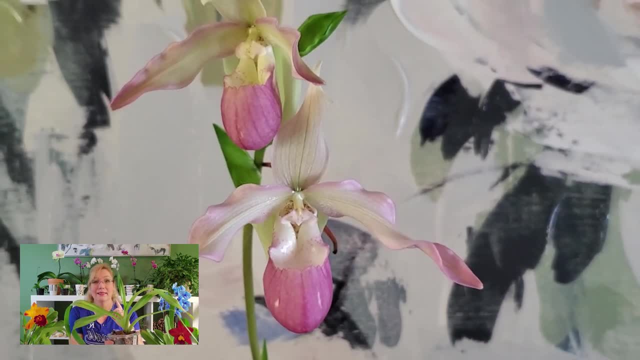 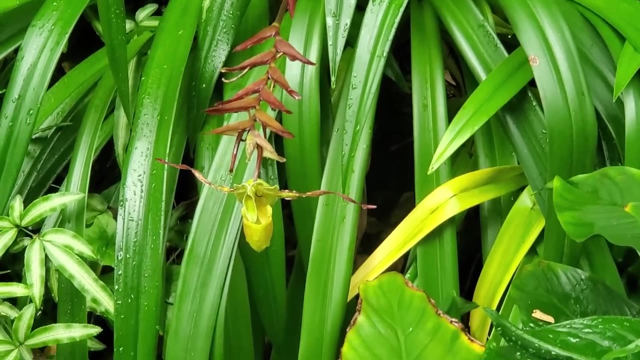 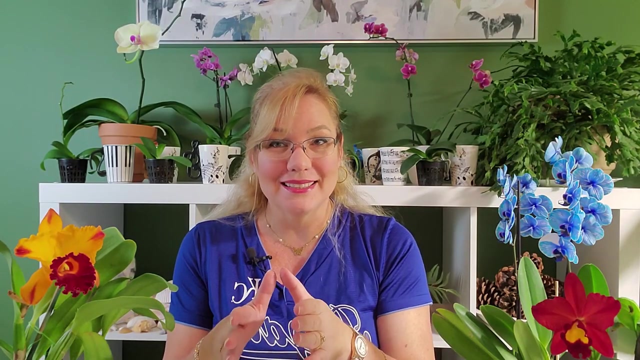 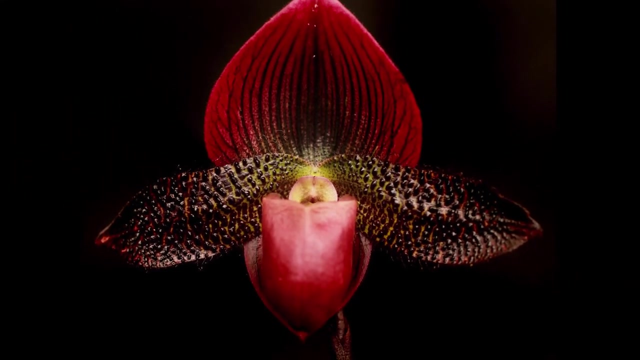 the stem is closer and they are terrestrial orchids. They grow in the soil. These you can commonly find around United States in wetlands and wooded forest. The pathiopedilum gets its name because of the distinct flower, This part of the lip. again, the lip is what mostly identifies. 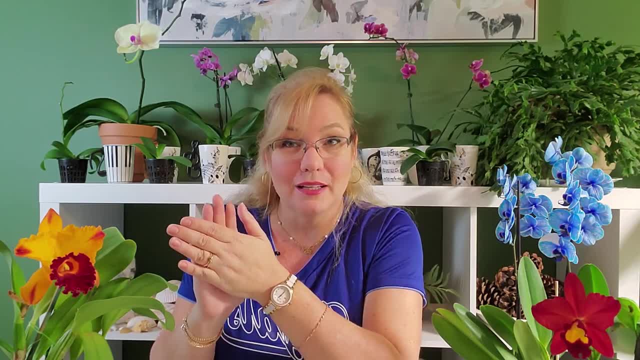 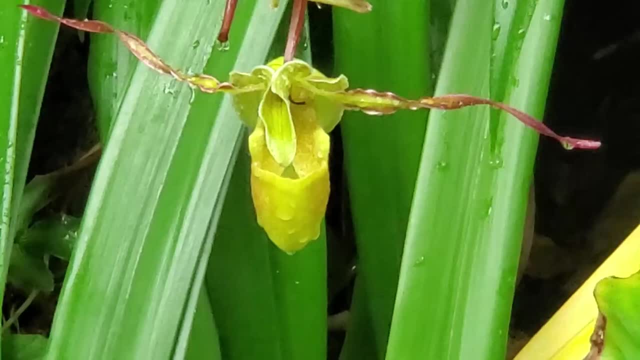 orchids. when they're in bloom, The lip of the pathiopedilum will steep down and then it will circle back up to form like a slipper or a moccasin. The name around the lady, slipper orchids, is extremely rich in culture because it is about an Indian girl. 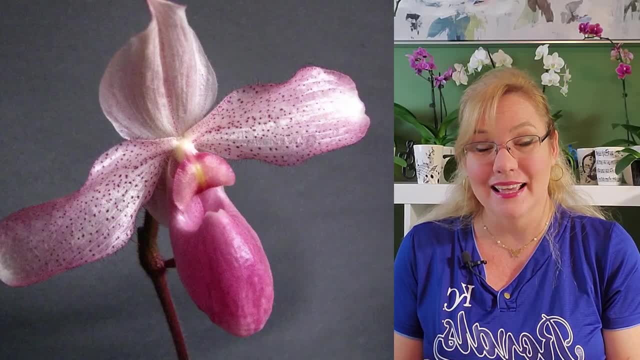 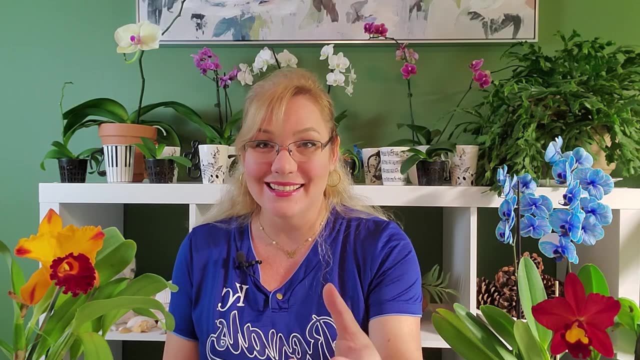 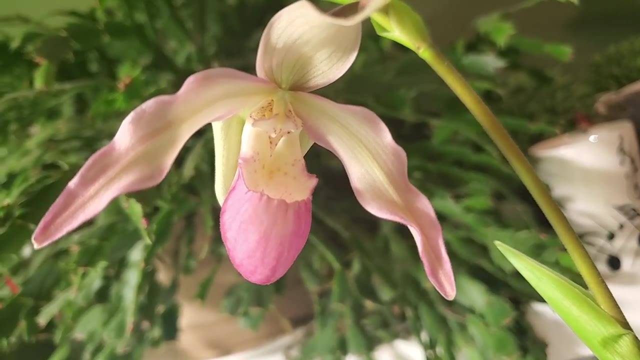 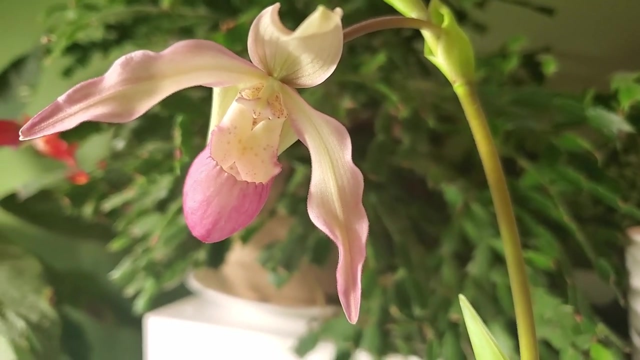 whose tribe gets plagued by a disease, and so she has to leave her tribe. and she travels through these horrible adventures to try to get a a cure for this disease. When she finds it, she travels back, but she leaves. She loses her slippers on the way, but it's in the dead of winter, so her feet start to bleed out and 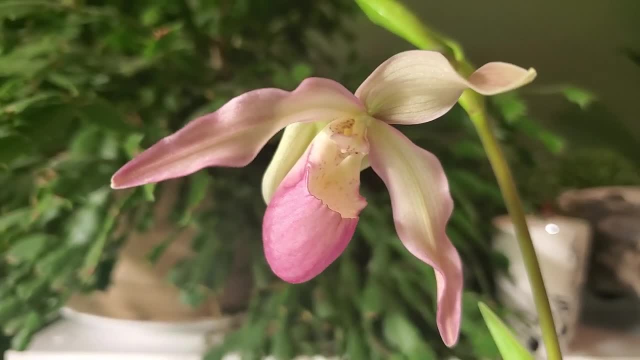 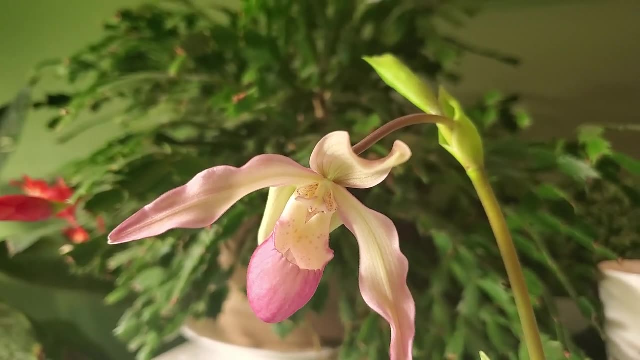 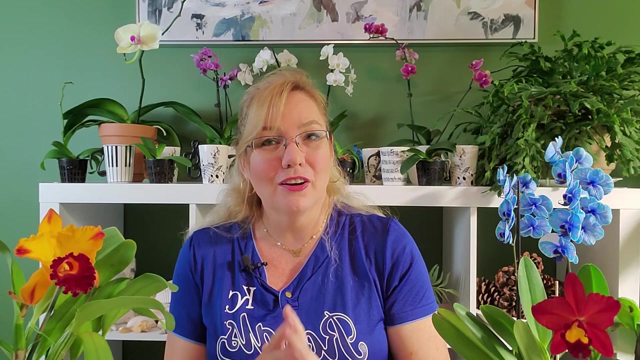 wherever she stepped on that trail trying to find the cure, would grow out a pathiopedilum which the Indians would call a moccasin. We took the moccasin and just called them lady slippers and from that reason on it's called lady slippers. but they are not only pathiopedilums: Lady slipper orchids. 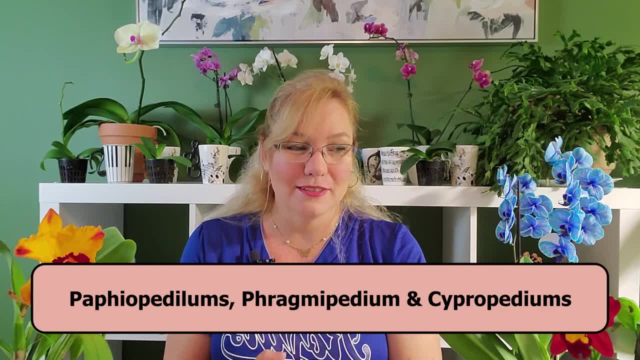 do also include fragmentary slipper orchids. The only thing that they do include fragmentary slipper orchids is the panty and then the lip of the pathiopedilum. Lady slipper orchids are also really big, and there are many other types of plant species. 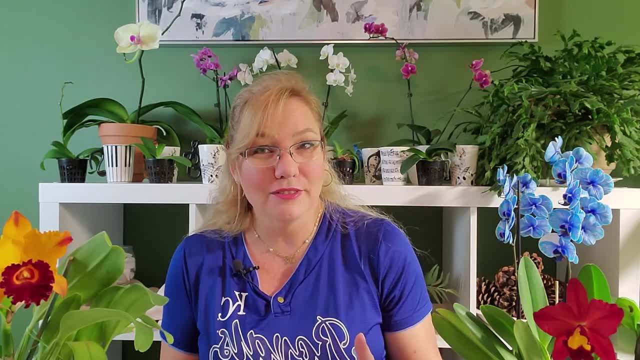 such as fr presup�iples, which can be found in over 100 years, such as acorns and a lot of other plant species, such as aphids- I mean a lot of plant species- and several other cockatiels or orchids and a lot of others.